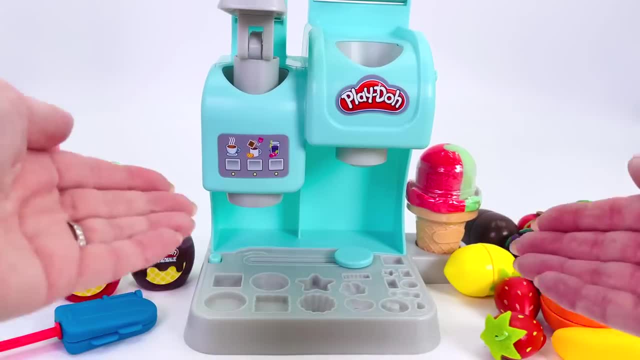 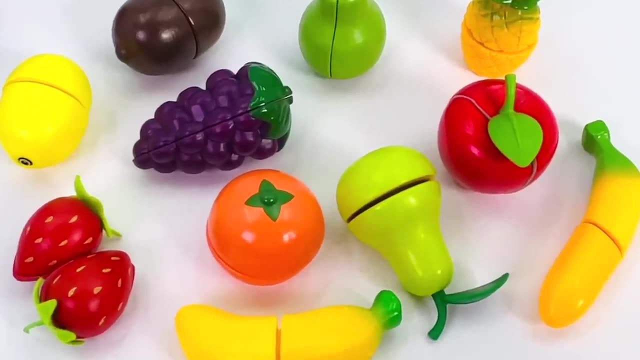 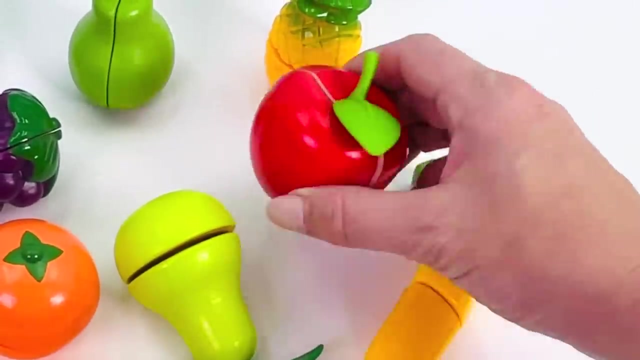 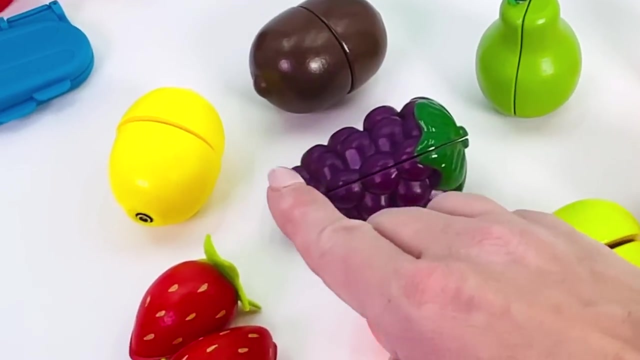 Wow, it's going to be a busy day today. I have lots of customers. Here's our first customer. She would like a strawberry ice cream sundae. Now, strawberries, when ripe, are the color red. Can you find a red fruit? Here's a red fruit. Hmm, but that's an apple. Let's go look for the strawberries. Can you see them? Oh, they're. down here on the left We have two strawberries. 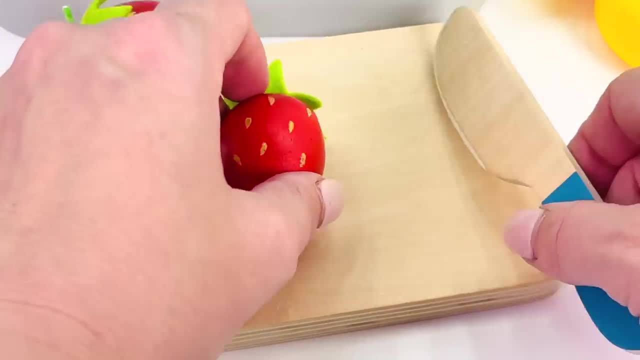 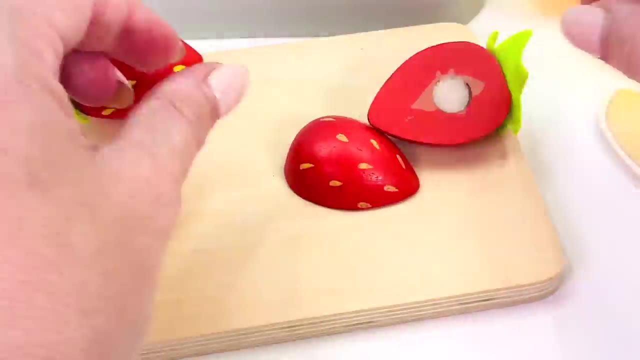 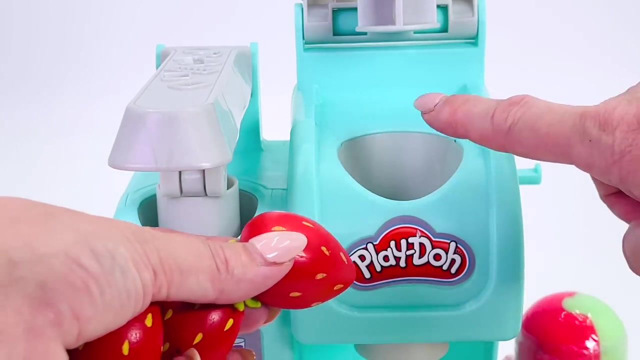 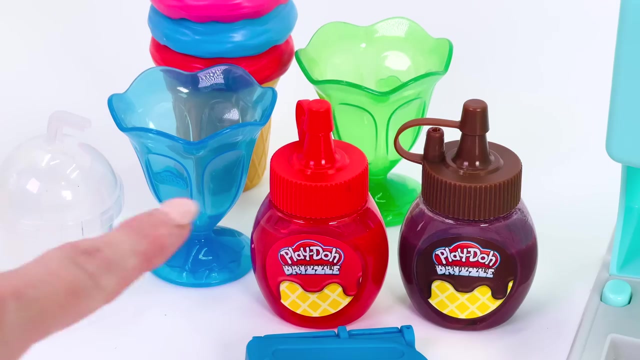 Let's go prepare them. I'm going to cut them in half. Here's one strawberry. I've cut it into two halves And here's the second strawberry. Now I can put the strawberries into my toy ice cream maker. That's one, two, three and four. Hmm, I need a cup to put the ice cream into. 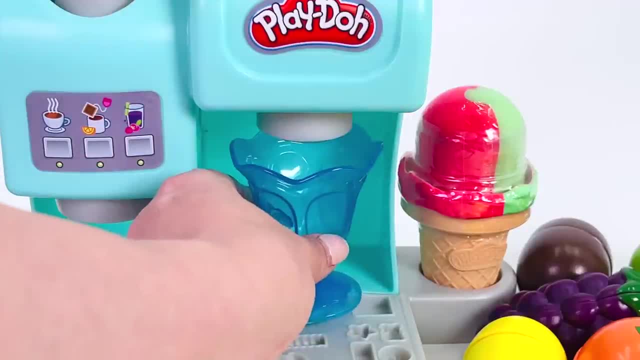 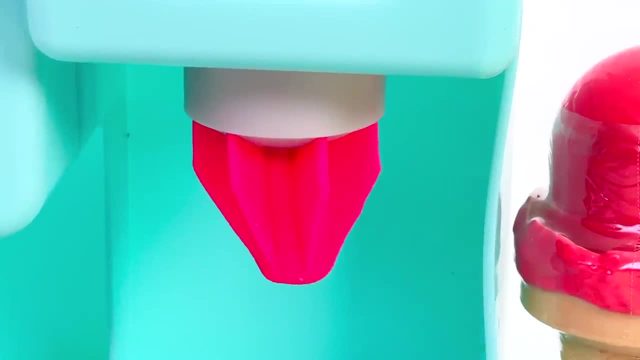 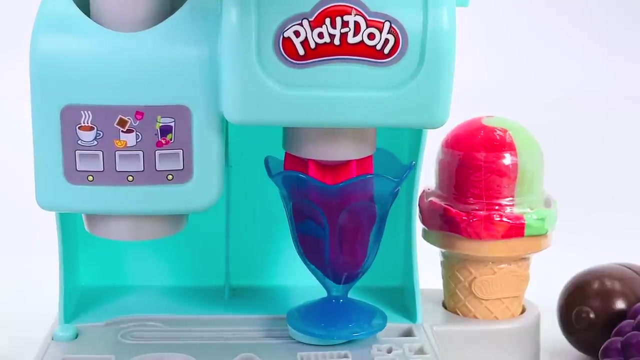 Let's go do it. We'll use this blue one, Put it under here, Push the lever down. Oh, can you see something coming out? Oh, look at that. Wow, The ice cream is coming out of the machine. Oh, I can't wait to serve this up to the customer. 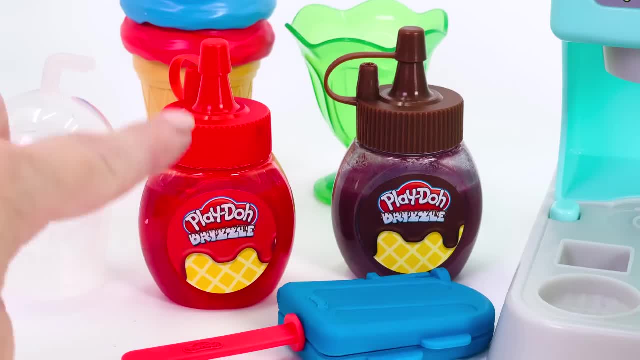 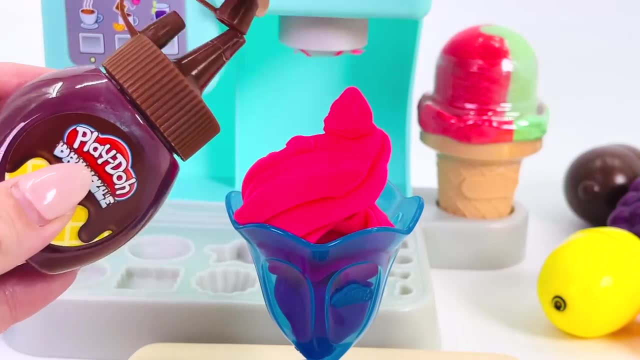 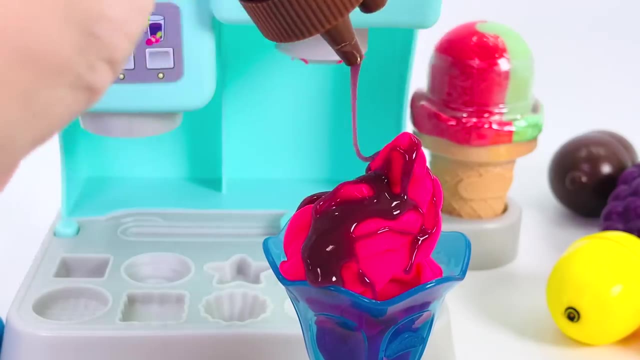 Hmm, but it's not quite ready. I think I'll put a topping on this strawberry and strawberry ice cream. Oh, and chocolate. How about this chocolate one? I'll just drizzle it on here. Oh, that looks about right. And what else? Oh, I have these fruit. Hmm, what shall I pick? 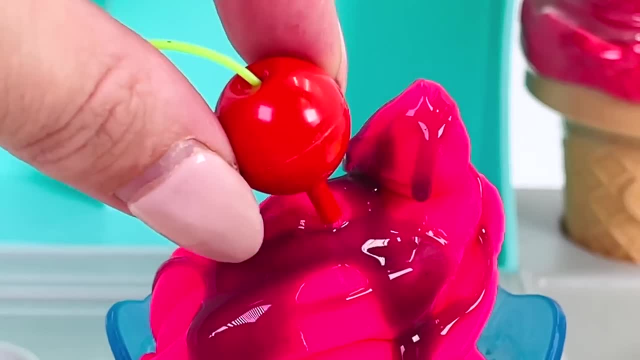 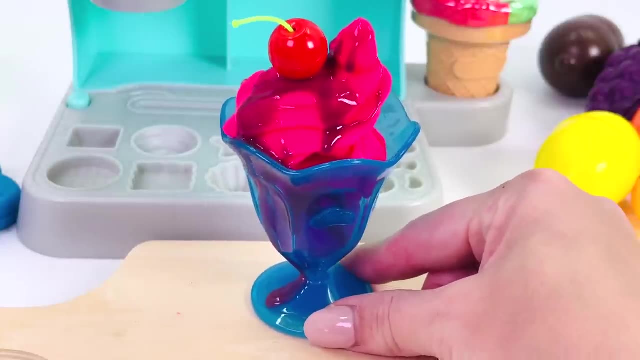 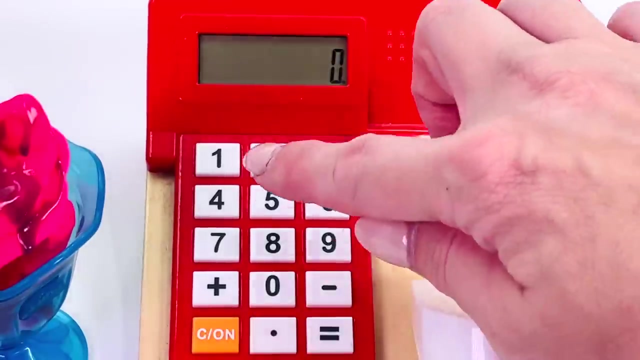 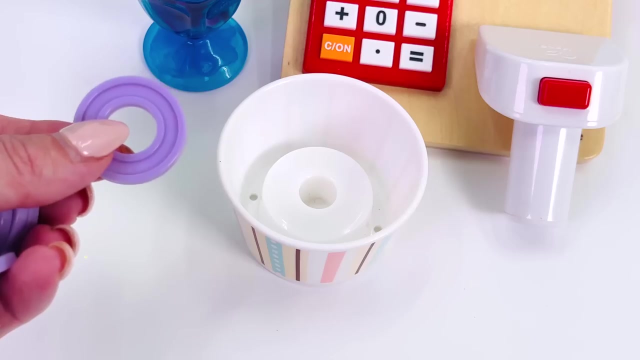 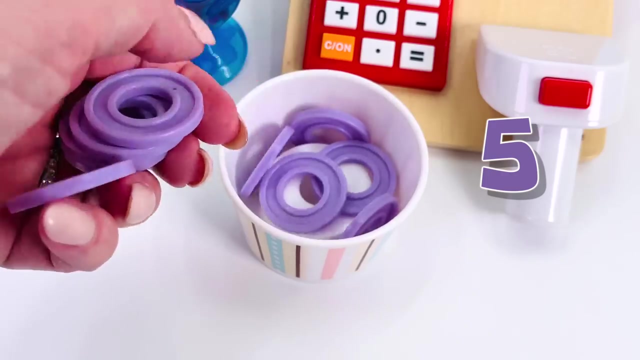 How about this bright red cherry garnish? I think I'll put it right here. Looks great, Let's go serve it up to our customer. The ice cream sundae costs ten coins. A customer has given us all these coins. Let's count them together. That's one, two, three, four, five, six, seven, eight, nine and ten. Great counting. 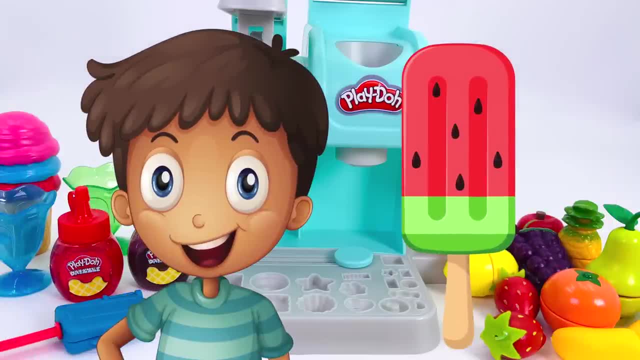 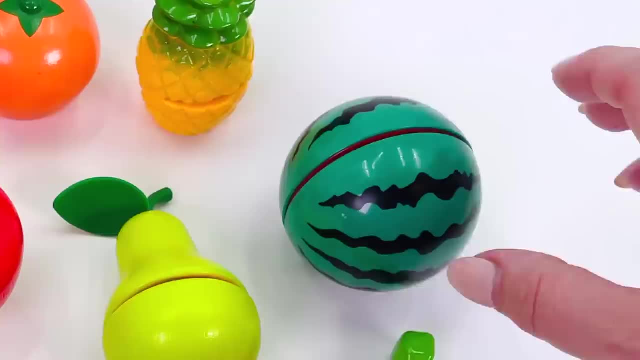 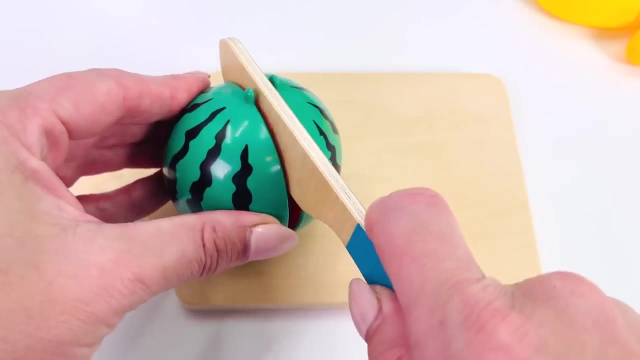 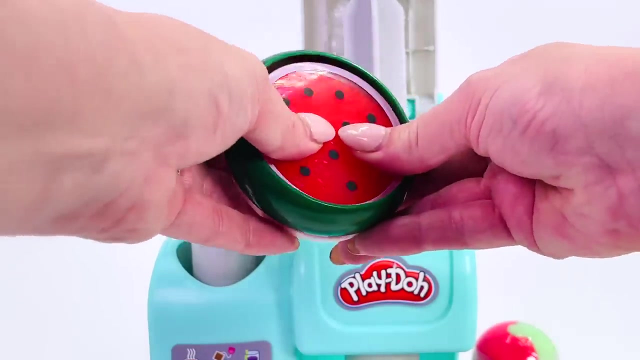 Here's our next one. Here's our next one. Here's our next customer. He would like a watermelon popsicle. Can you help me find the watermelon? Here it is. Hmm, it's green on the outside. Let's slice it and see what it's like on the inside. Oh, it's bright red. Let's go add it to the ice cream machine. 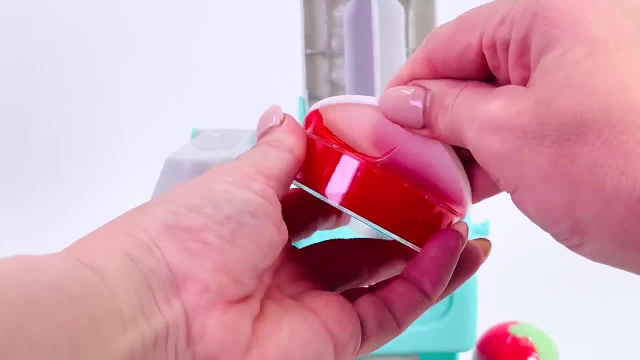 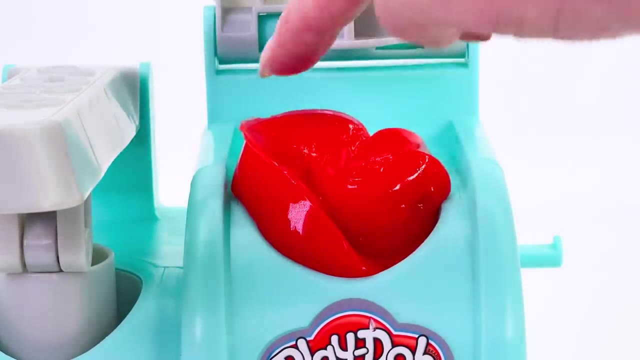 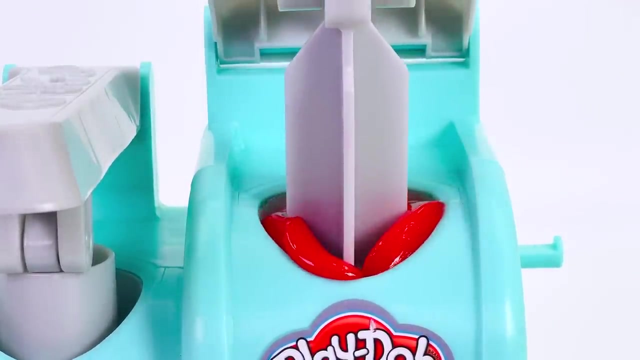 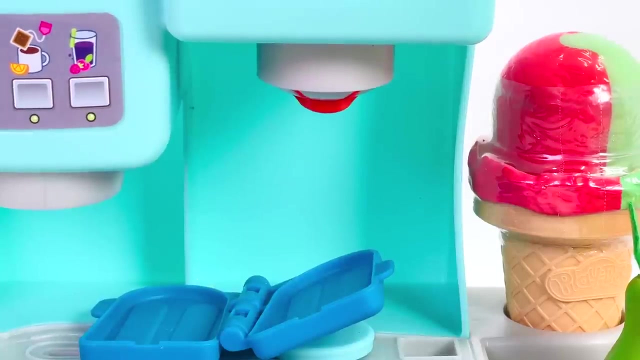 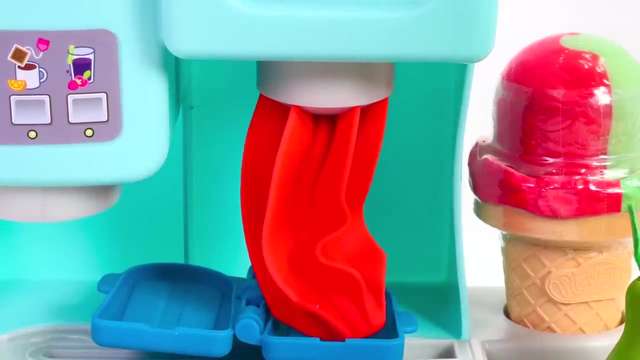 Here's our next one. Oh yeah, Just put it in here. Ooh, it's all sticky and gooey. And push the lever down, Here we go. I have my popsicle mold. I'll just put it under here. Oh wow, It's bright red And now it's turning green. 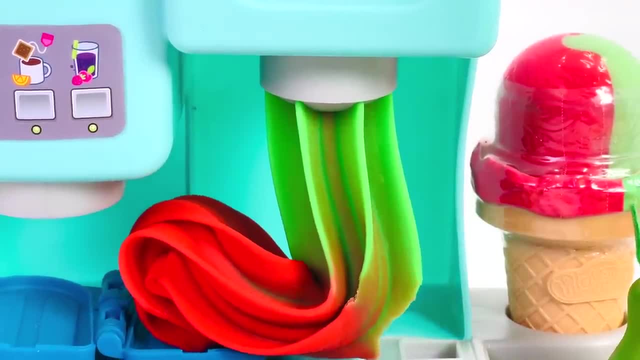 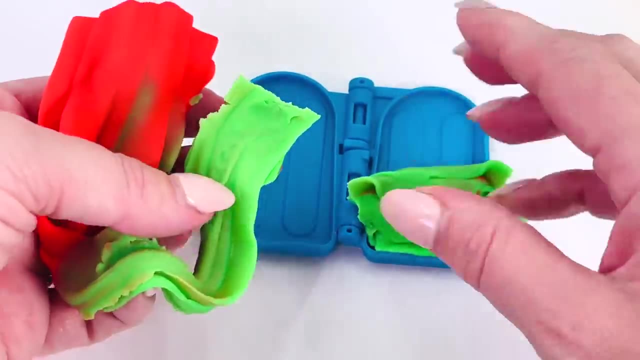 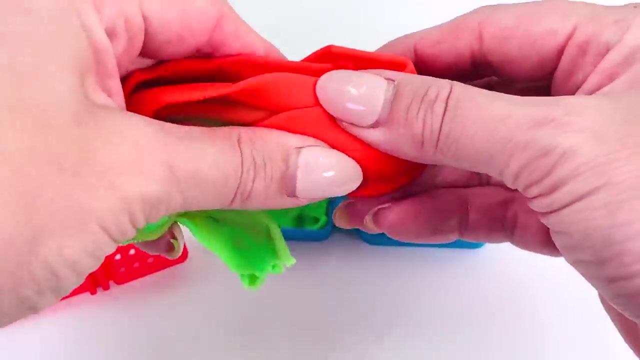 Oh wow. It's all sticky and gooey And now it's turning green. Nearly done. Now let's make a popsicle. Watermelon is usually green on the outside and red on the inside. I'll place the green here at the bottom and some red at the top of the popsicle. 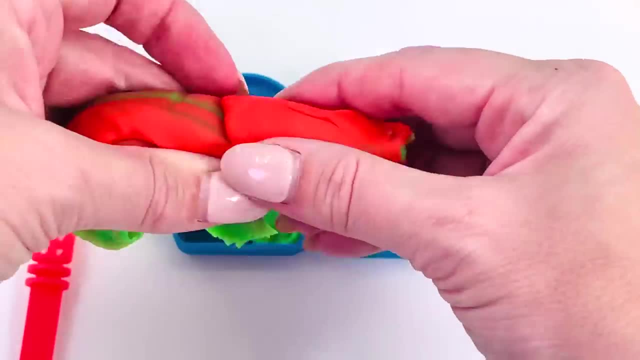 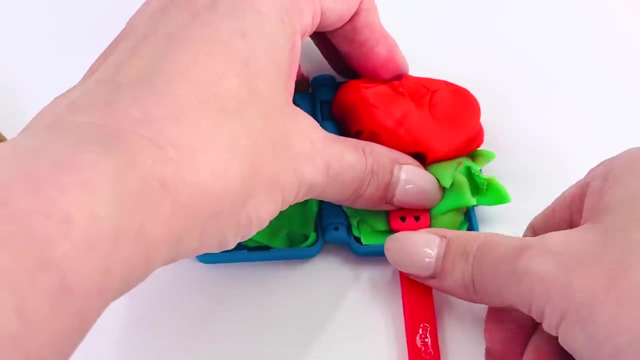 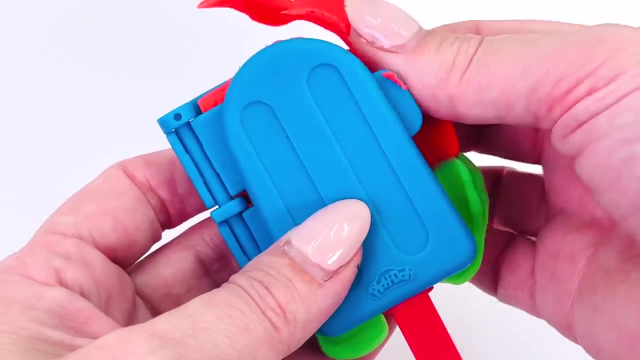 Just press it down here And one over here on the left. I have this red popsicle stick that I'll use. This will look nice And now I need to press it together firmly, remove the extra Play-Doh around the edges and now reveal the popsicle. 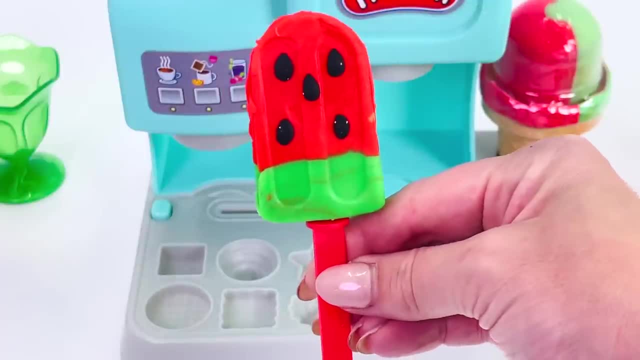 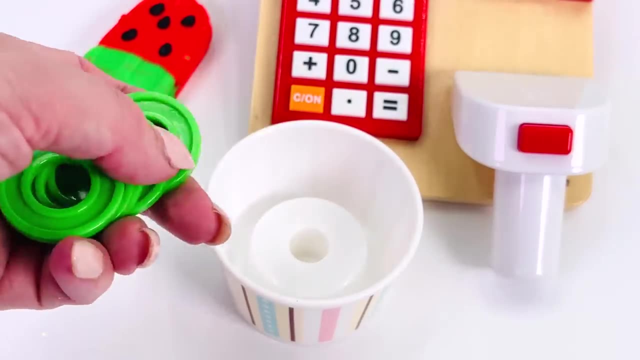 Oh wow, One watermelon popsicle. Let's go serve it to the customer. How much did it cost? Five coins. Let's count how many coins our customer gave us. That's one, Two, Three, Four And five. 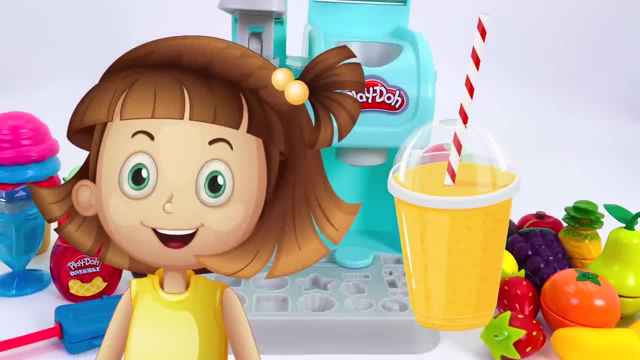 We've got another customer. She would like a banana smoothie. Can you find a banana? Hmm, it's a color yellow. Here it is. We've found it already. It's a banana. Let's go slice it. I think I'll use this piece here. 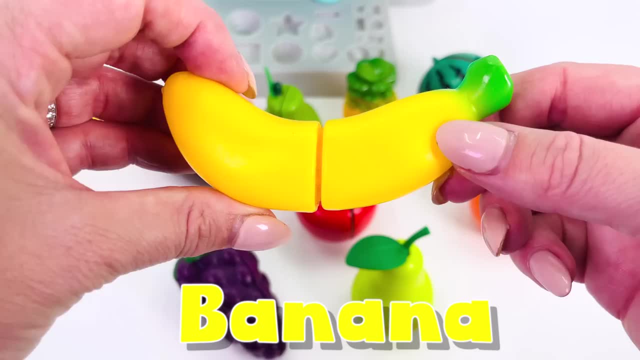 Pop it in the machine, Add some milk- Ooh, that's a good one. One, two, three, Oh wow, It looks like a banana. That's good. Now let's slice it. Ooh, that's a good one. 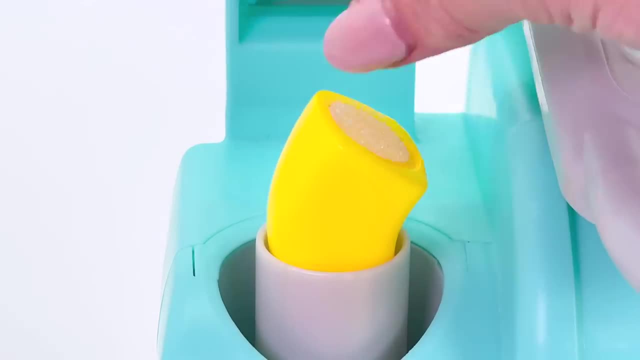 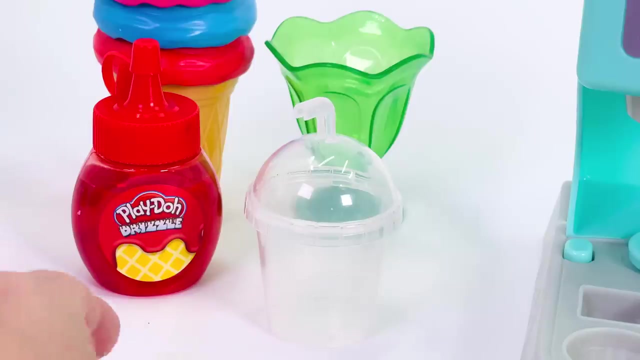 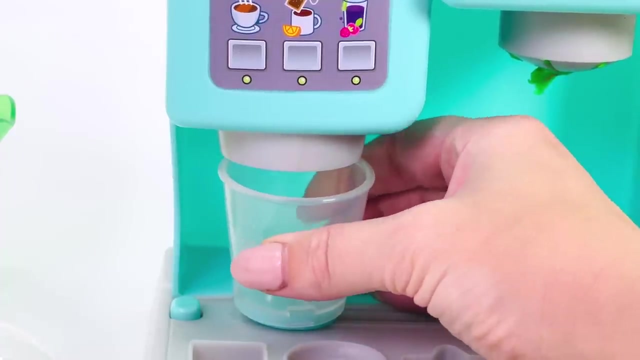 Three, Four And five. Oh wow, That's a good one. Three, Two, Three, Four, And I've got the smoothie cup. This will do Place it here. And which one's the smoothie? That's tea. 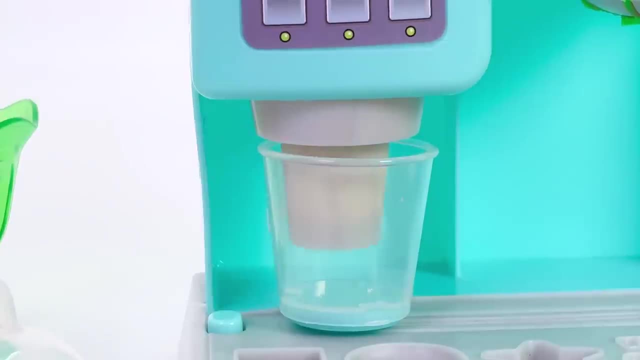 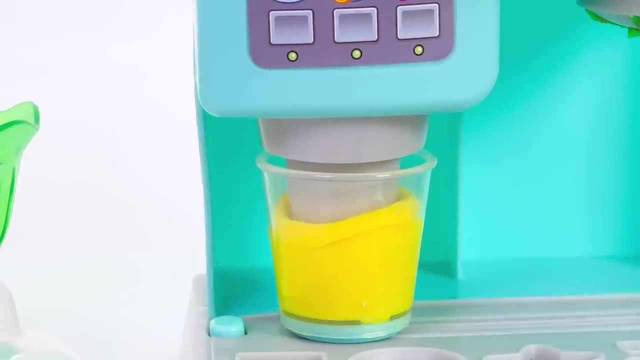 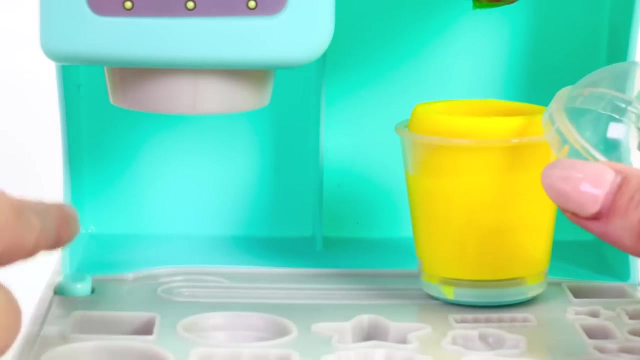 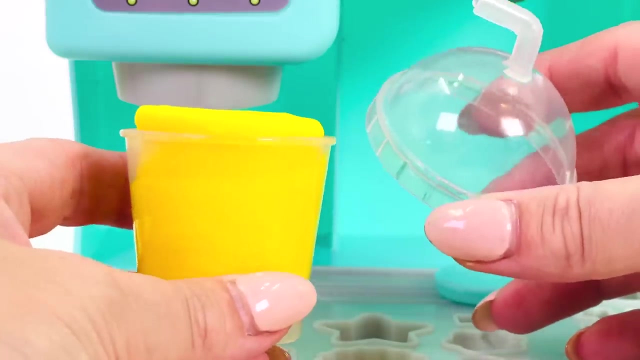 Oh, here's the button. Press the button, Here we go. Whoa, look, It's all yellow banana. Here's my lid. I'll just press the button, Here we go, Place the lid on firmly And serve it up to our customer. 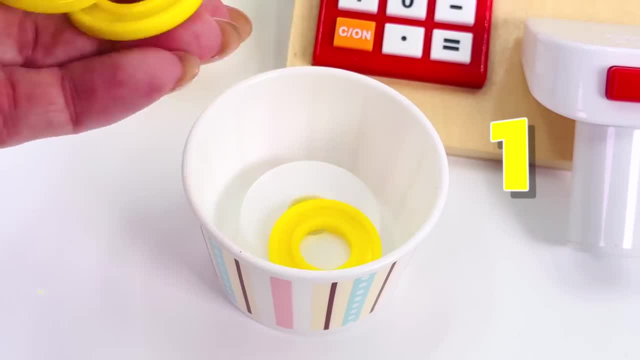 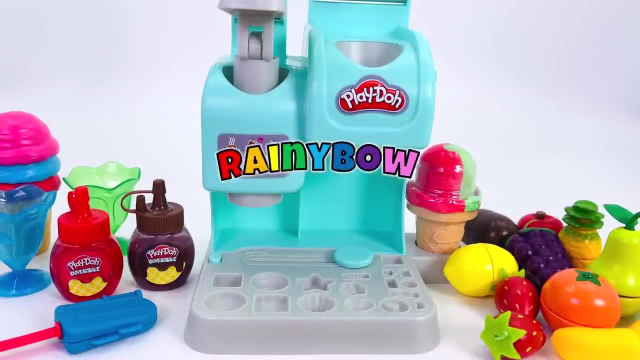 The smoothie costs three coins. That's one, two and three. Wow, I had so much fun today in my toy kitchen. See you next time on Rainy Bow. Welcome to Rainy Bow Kitchen. Hello Chef, How are you? 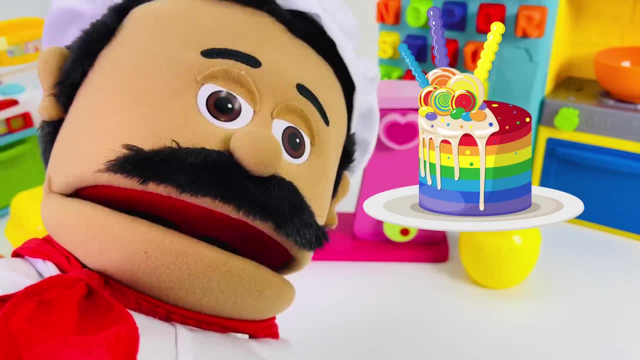 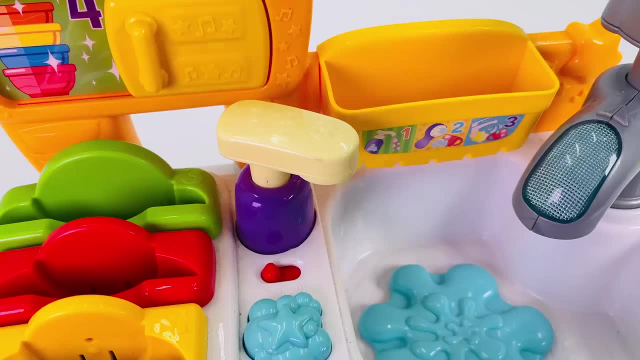 How can we help you? today? I need some help to make a surprise birthday cake. Sure, Let's go make the cake. Before we start to cook, we need to wash our hands. I'll use some soap And Oh water. 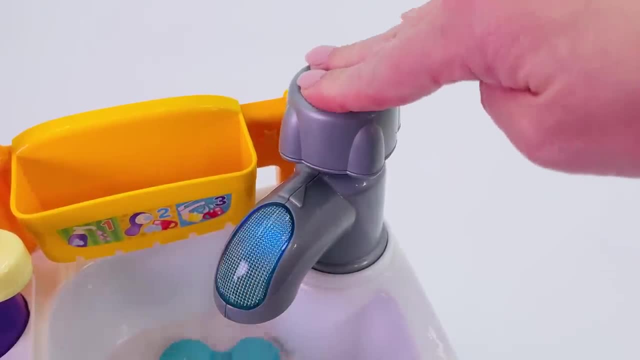 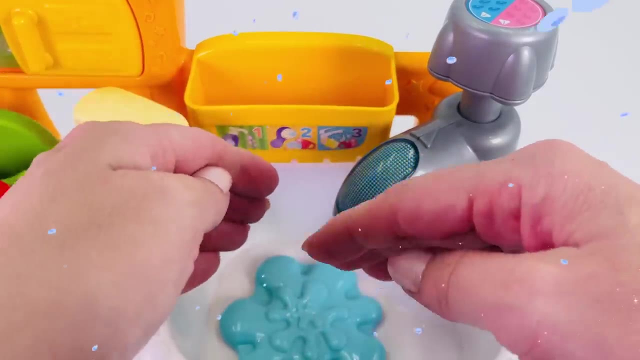 Cold water. We'll use the cold water. I'm mixing the cold water and the soap to get my hands really clean before I start to cook. What's the first ingredient? Flour. What's next? Sugar. The flour and sugar are dry ingredients. 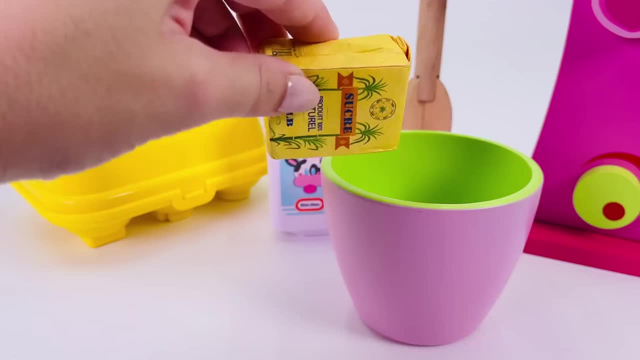 Now I need to add the wet ingredients. Here's a carton of milk. Whistle it off And pour it into the bowl. Oh, and don't forget the eggs. I have this carton. How many are in there? There's six all together. 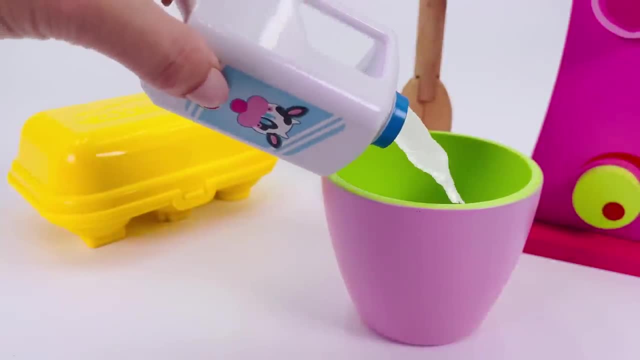 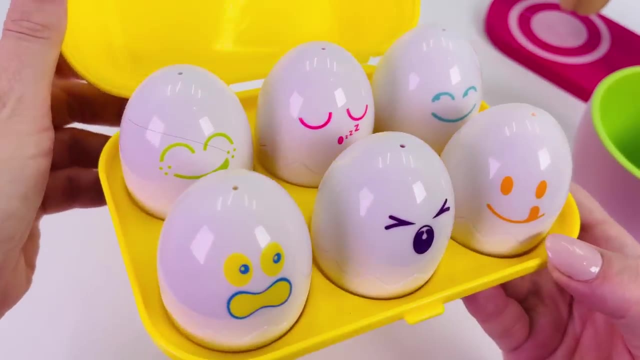 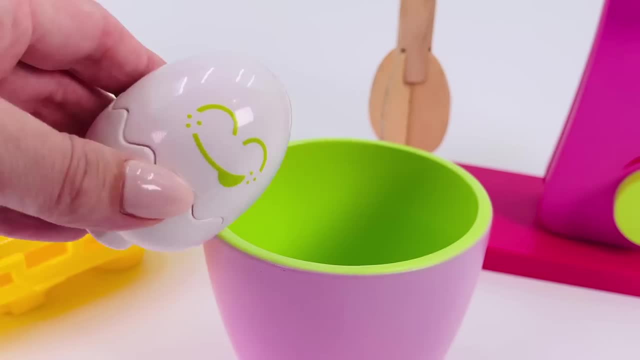 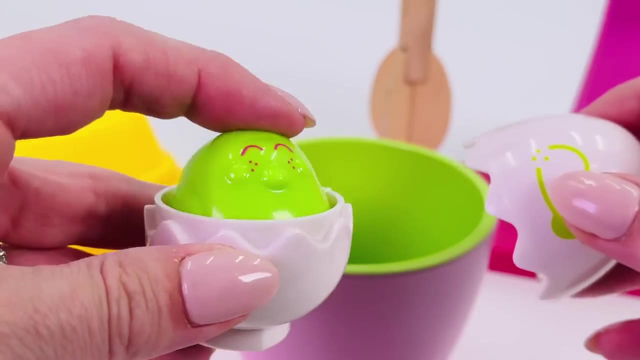 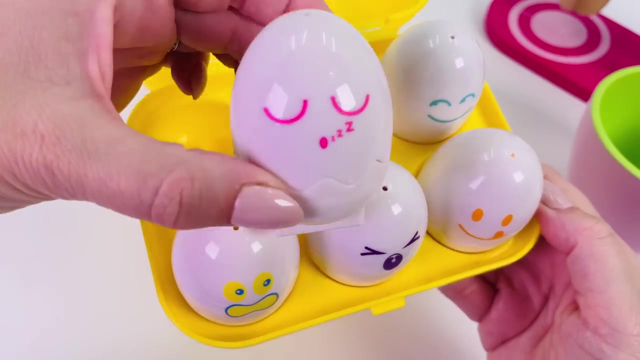 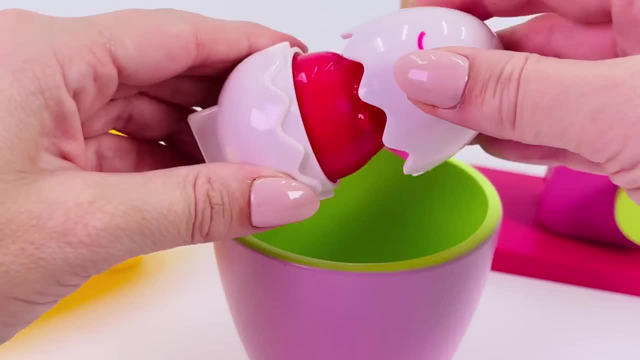 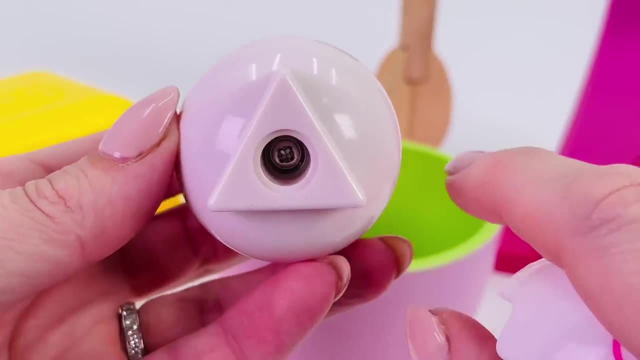 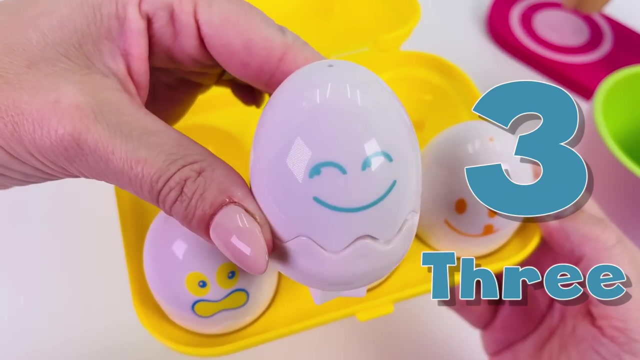 Oh, I can't wait to see what color's inside. It's the color pink, Pink. And what's the shape on the bottom? It's a triangle. Here's our next egg. Here's our next egg, Egg number three. 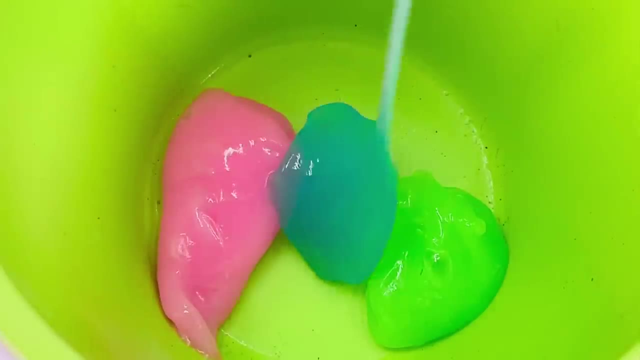 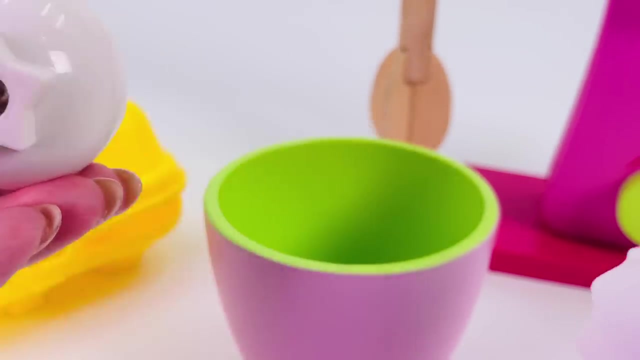 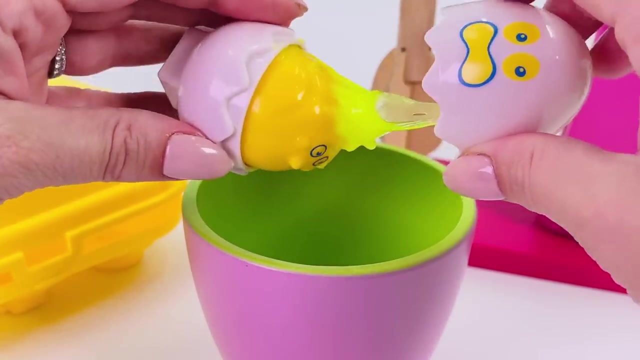 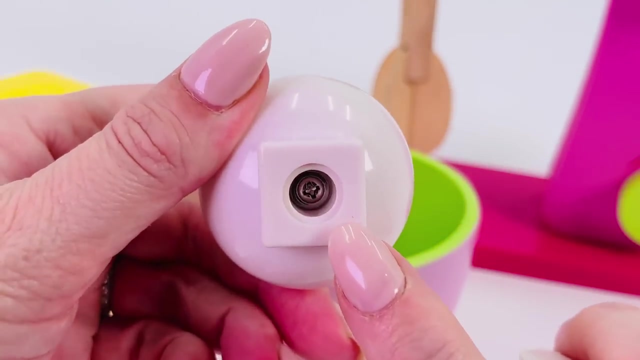 Ooh, it's all gooey. Egg number three is the color blue And it's got a star on the bottom. Egg number four looks a bit scared. What color is egg number four? It's the color yellow, And what shape is it? 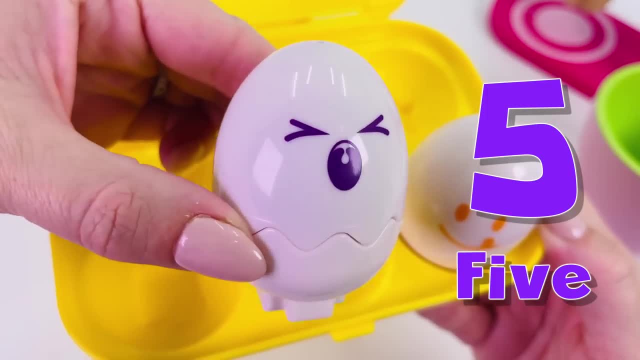 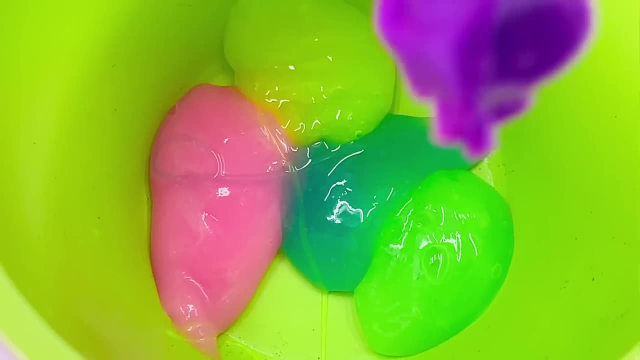 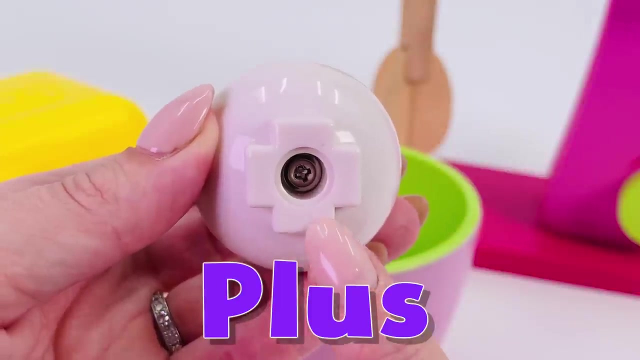 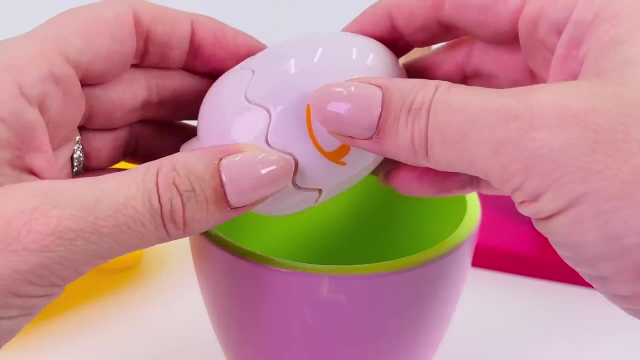 It's a square. This is egg number five. Ooh, Egg number five is the color purple And it has a plus sign on the bottom. We only have one egg left. It's egg number six. Let's add it to the mixture. 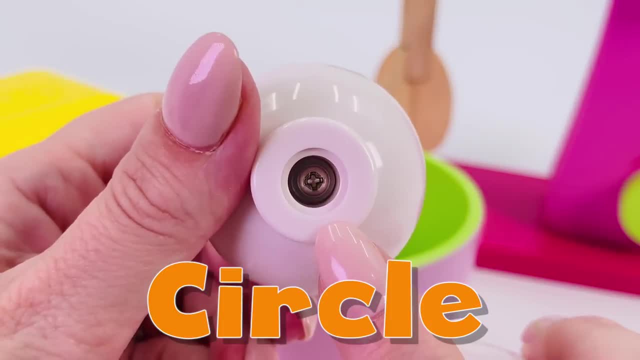 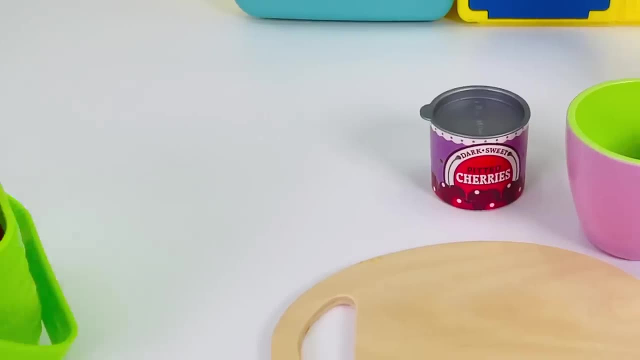 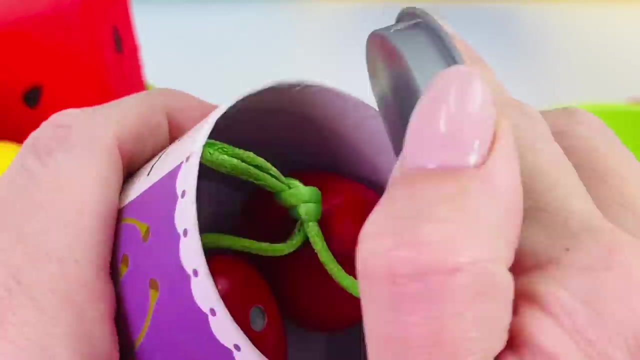 Egg number six is the color orange And it has a circle on the bottom. Ooh, look at all the egg mixture in there. Okay, now I need to add some fruit. I have a can of pitted cherries. Let's add it to the mixture. 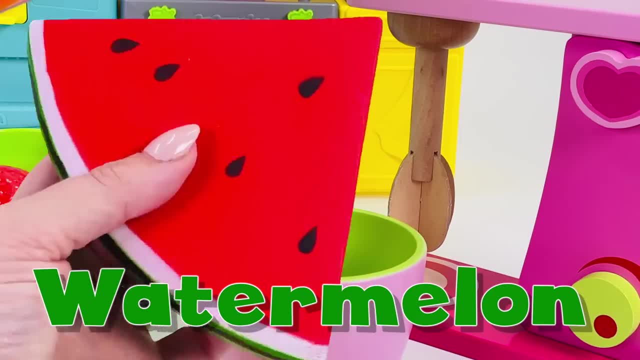 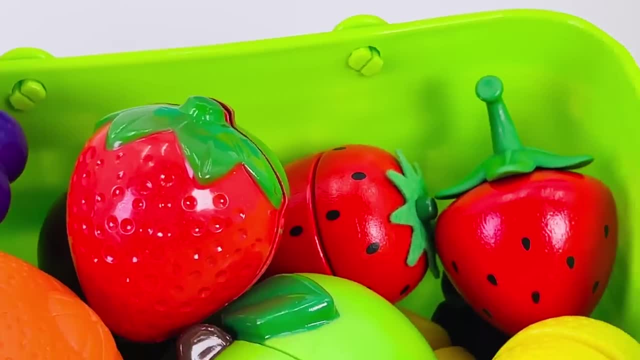 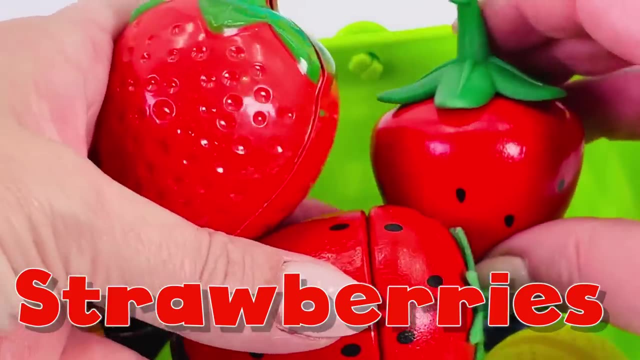 Oh, look at this juicy watermelon. I'll just squeeze it a bit to get off the juice. That's about right. Hmm, Oh, I know I have these ripe strawberries. They're beautiful and red. First, I need to wash them under the faucet to get them clean. 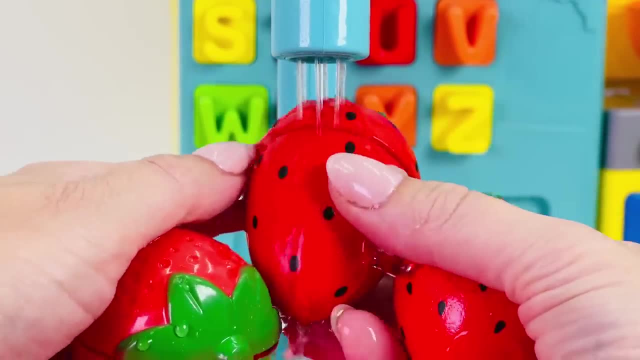 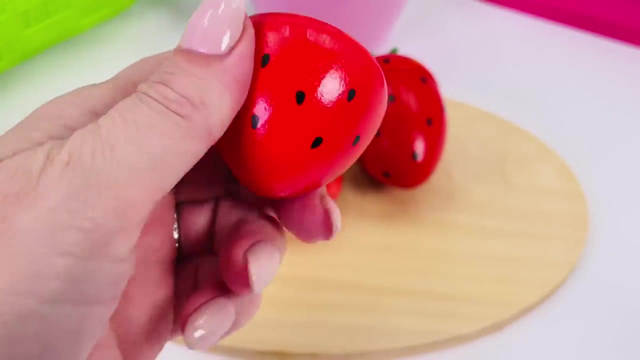 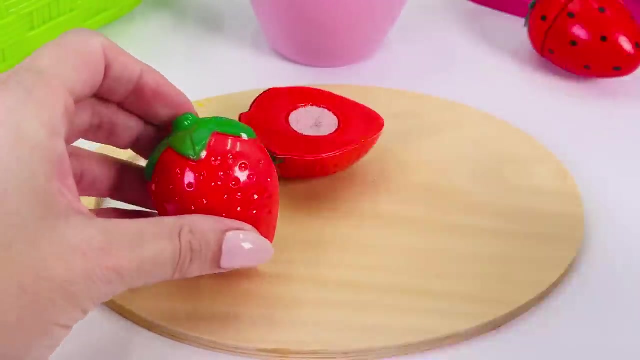 Oh, these will be great in the rainbow cake that I'm making: All done, Nice and clean. Oh, these will be great in the rainbow cake that I'm making: All done, Nice and clean. stick the stalk off this one. We don't need that, And I'll cut this one in half. There's 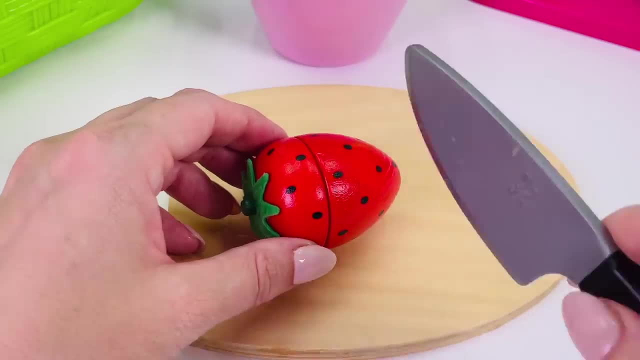 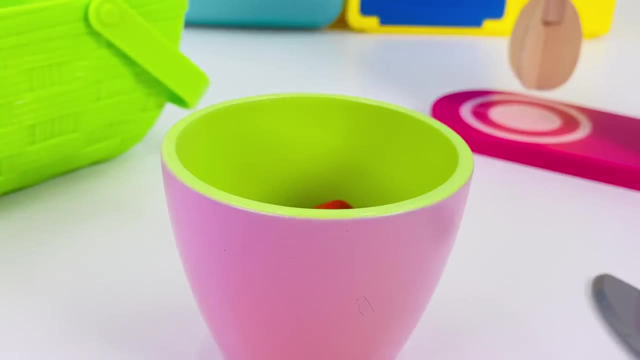 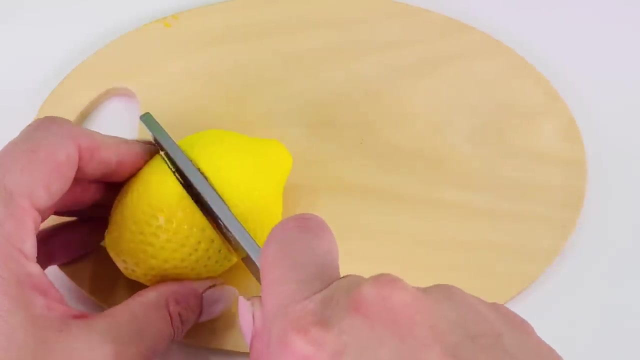 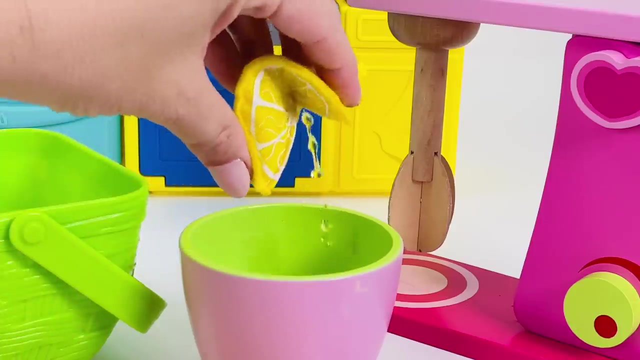 two halves, One half and two halves, And cut this one in half, also One and two. What's next? Oh, how about this lemon? Let's cut a slice. Oh, we have a wedge of lemon, Let's squeeze it into the mixing bowl. Oh, look at all the juice coming out. I think that's. 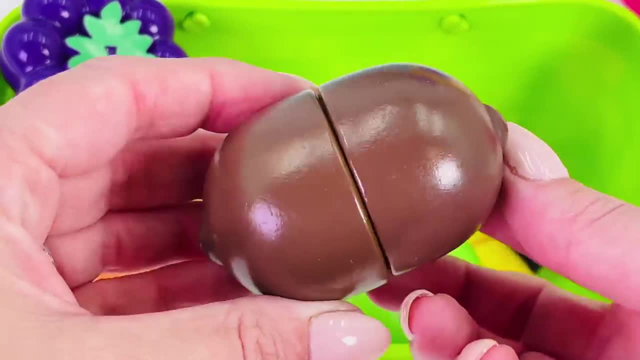 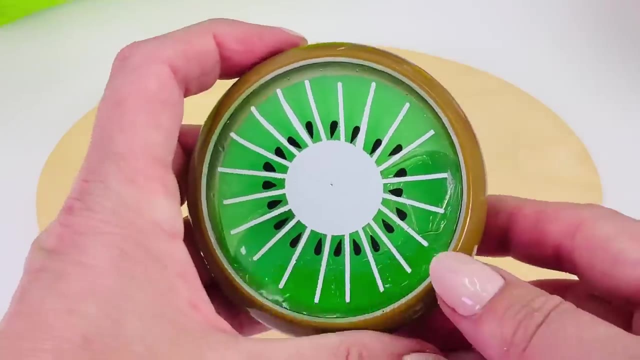 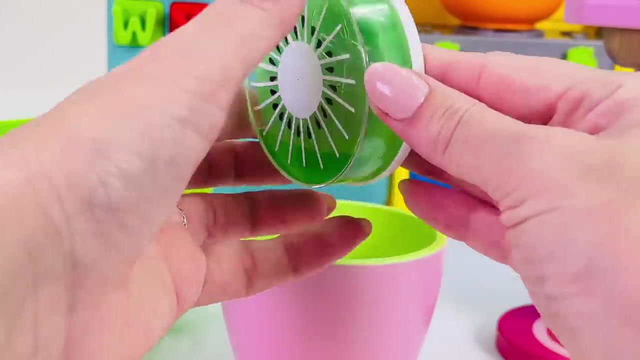 enough. Hmm, what's this type of fruit? It's brown and fuzzy on the outside and green on the inside. It's a kiwi. We have our slice of kiwi. What's next? Oh, how about this lemon? Now, let's go add it to the cake mixture. Oh, just look how green it is. We've added. 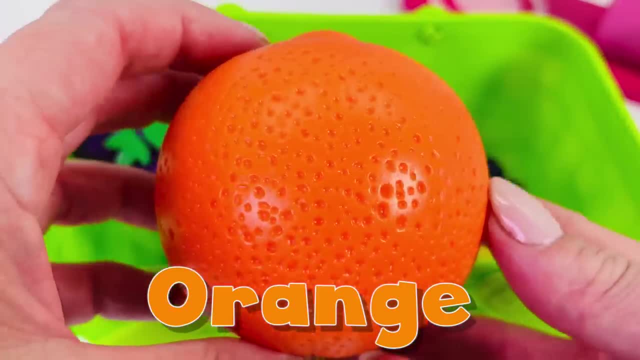 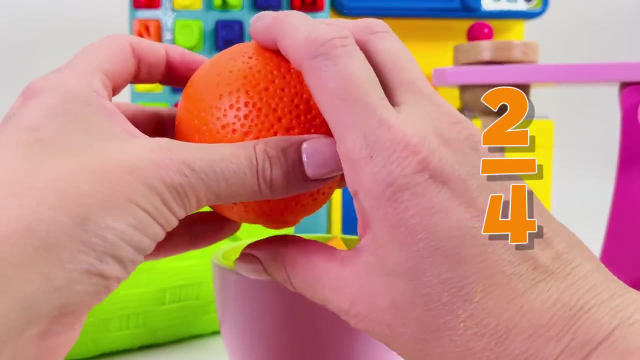 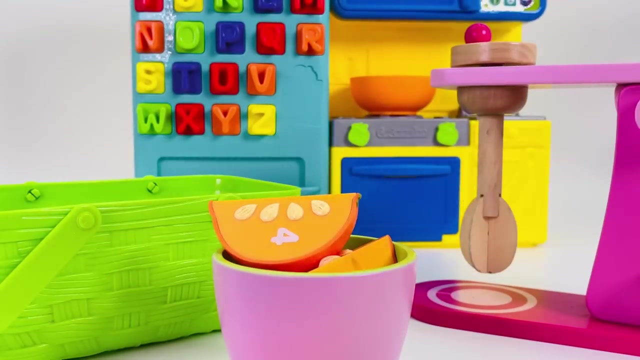 the kiwi. Now, what's next? What's this fruit? It's an orange. It's one quarter, two, three quarters and four quarters. We've added the kiwi. Now let's go add it to the cake mixture. 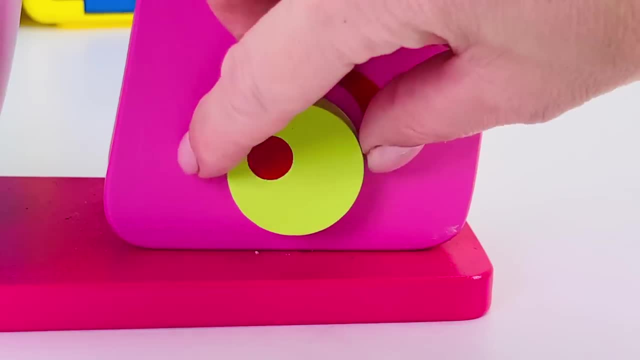 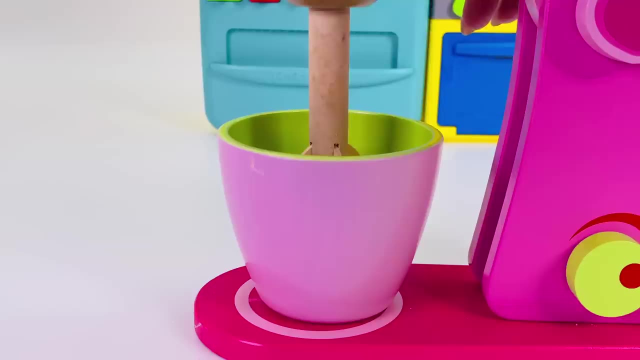 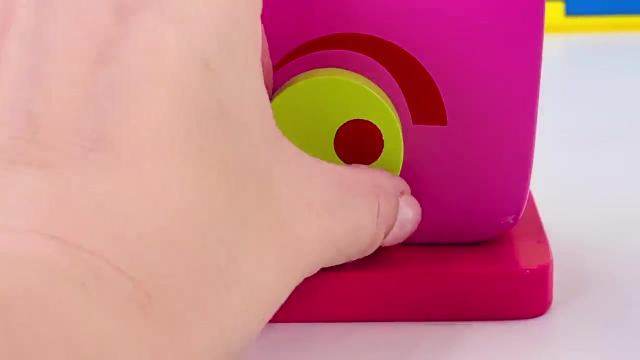 I think that's enough, And we've added all the fruit we need for the cake Now. all we need to do now is mix the ingredients together, Turn on the mixer, turning it around. Nearly done, All finished, Let's turn off the mixer. 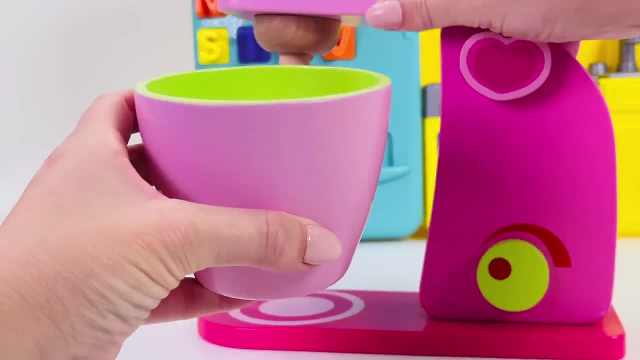 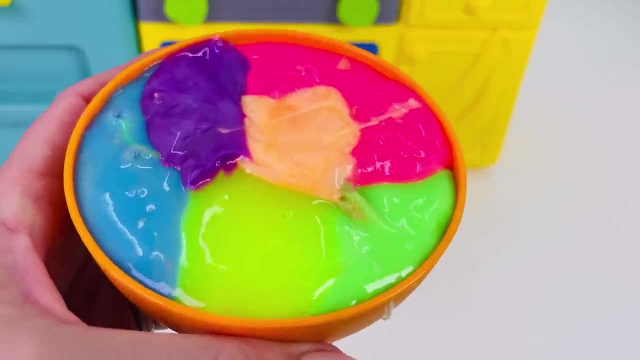 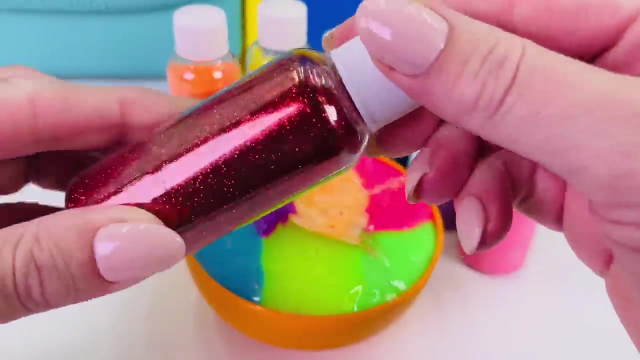 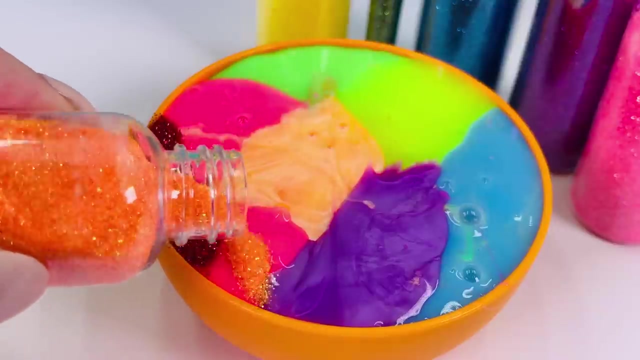 Now we've mixed the ingredients together, I'll add it to the bowl. Oh, look at it. It's all wibbly wobbly and it's so colorful. oh, how about i add some extra color? that's red now for some orange sparkle. 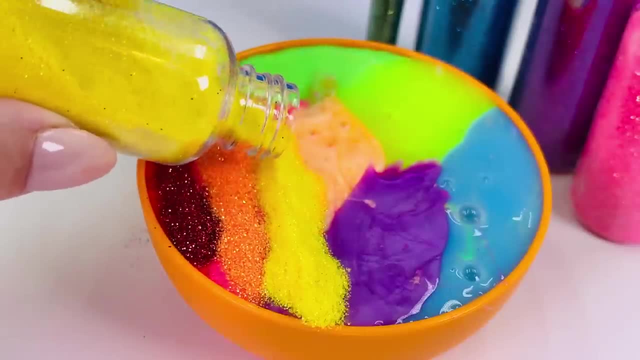 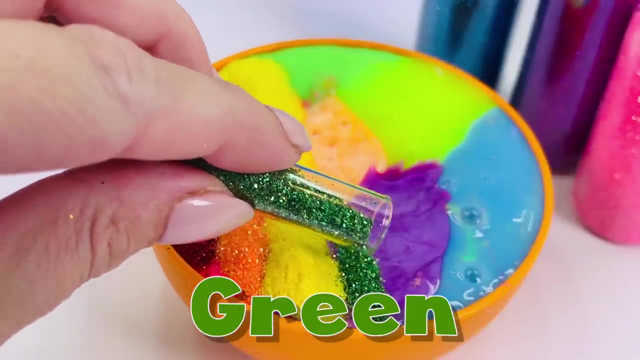 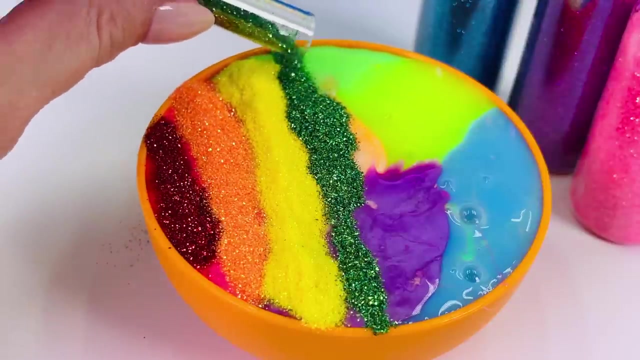 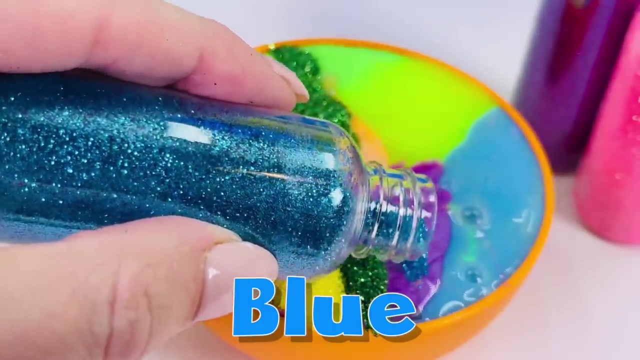 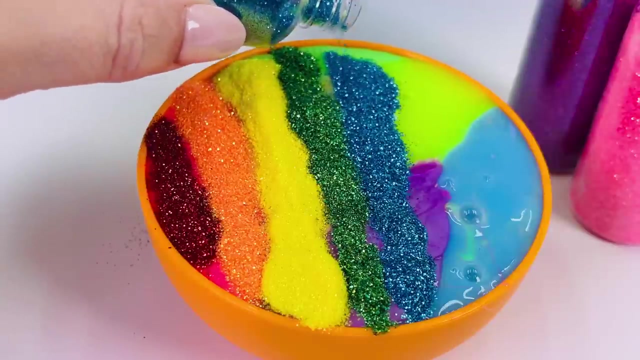 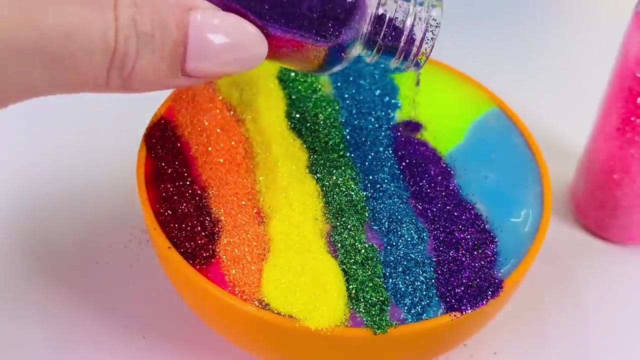 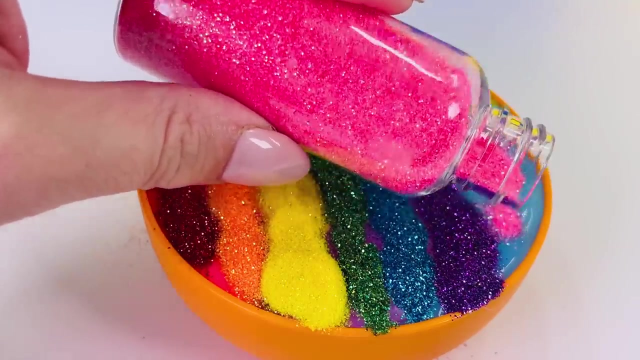 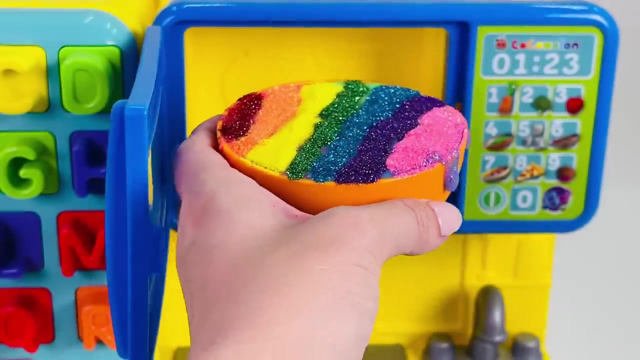 now i'm adding some yellow. what's next? how about some green? it's looking really pretty. this is going to be an amazing toy rainbow cake. next is blue, now purple, and last add a touch of pink- all done. oh, it looks so sparkly. all i need to do now is cook it in my toy microwave. 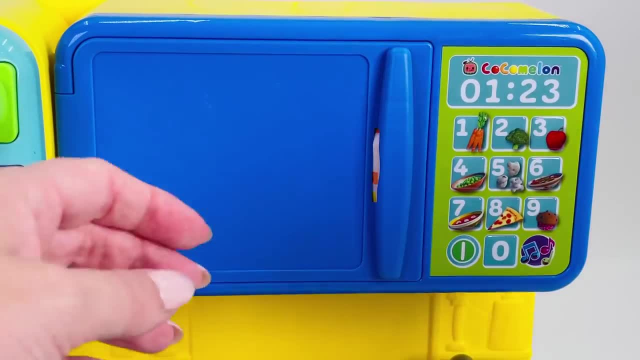 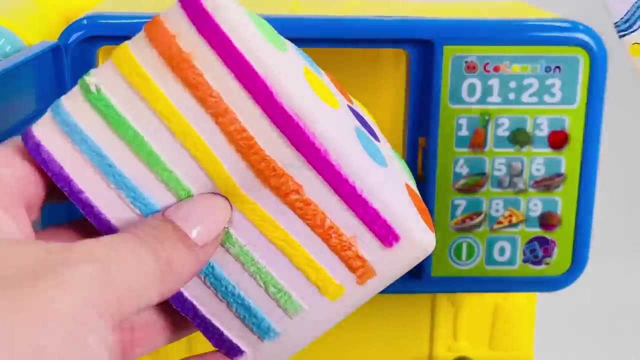 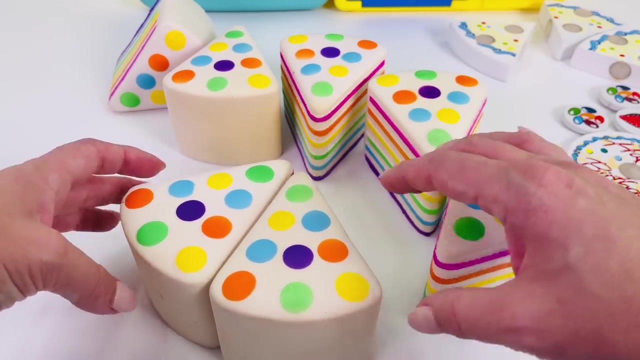 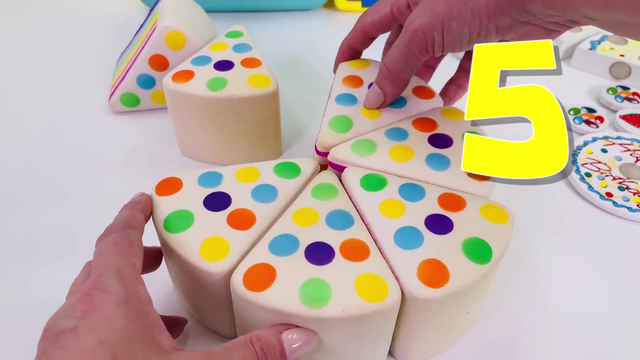 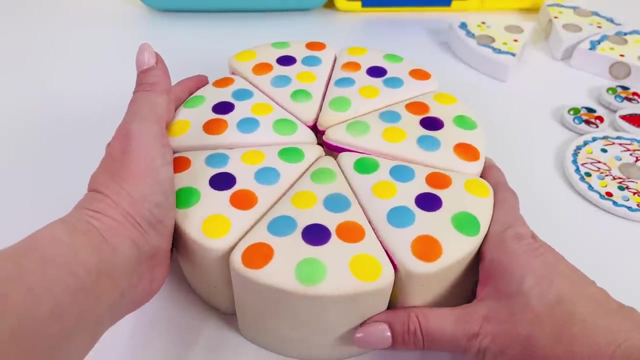 now what number was baking? that's right number: nine. did you hear that it went ding? i think it's cooked. let's go make the cake. here's one slice. that's two, three, four, five slices, six and seven. now i need to make the top layer. i have all these pieces. can you help me put them in my feet? 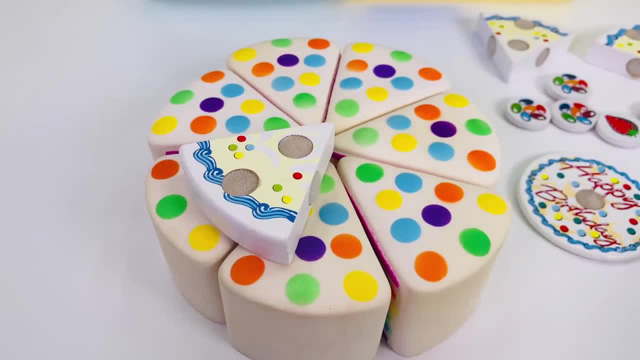 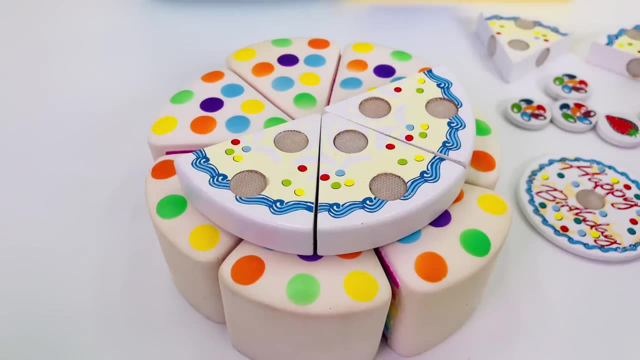 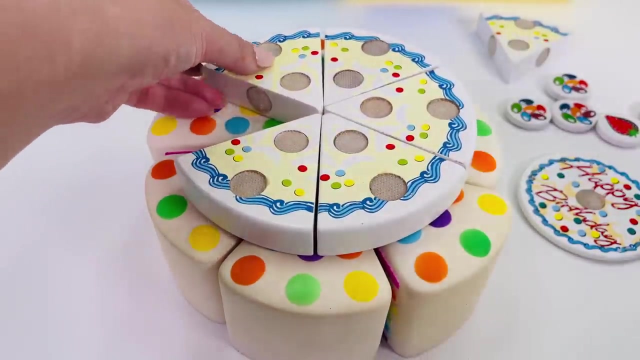 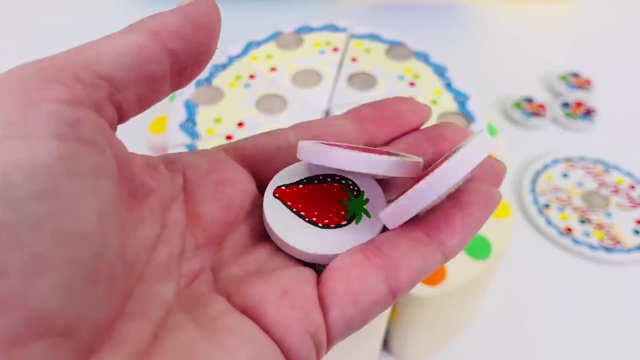 together. Here's one, two, three, four. Each wedge is the shape of a triangle, Five And all together they make a circle And six Great. Now we're ready to decorate the top. I have these three strawberries. Can you help me put them on the cake? Okay, I'll put one. 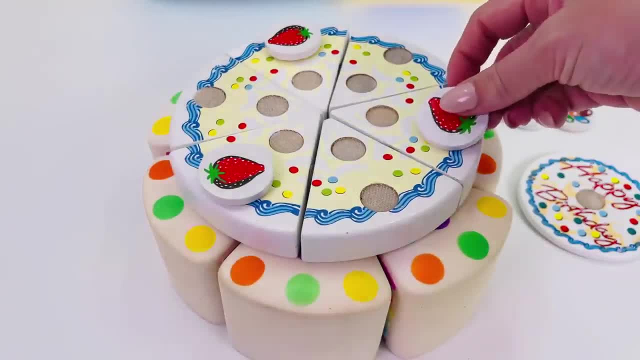 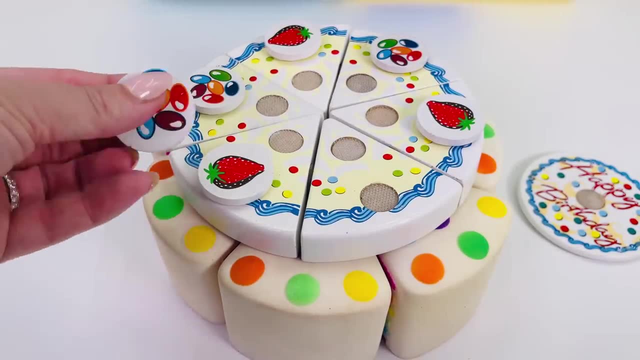 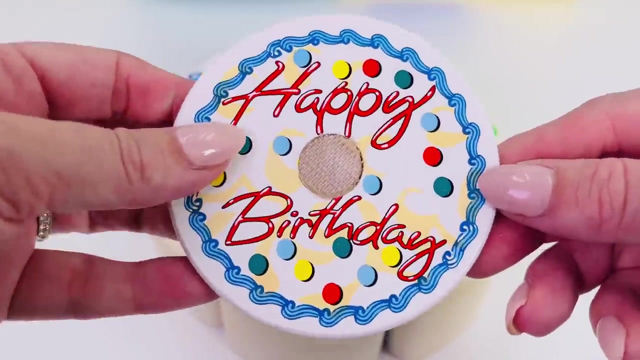 here, one down here and one over here on the right. And now for some jelly beans: One up here, one on the left and one down here. Oh, what's this? Oh, a special happy birthday sign. It'll go right here in the middle And a happy birthday.